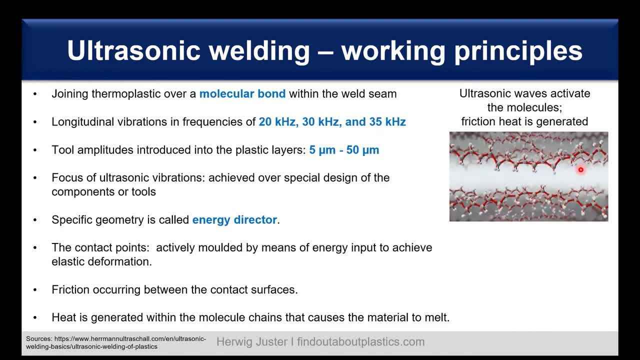 and this in turn generates heat which melts the polymers and then allows the joining. so we have as an input the different ultrasonic waves in different frequencies, such as 20 kilohertz, 30, 35 or even 40, and the. the amplitudes which are introduced in the layers are 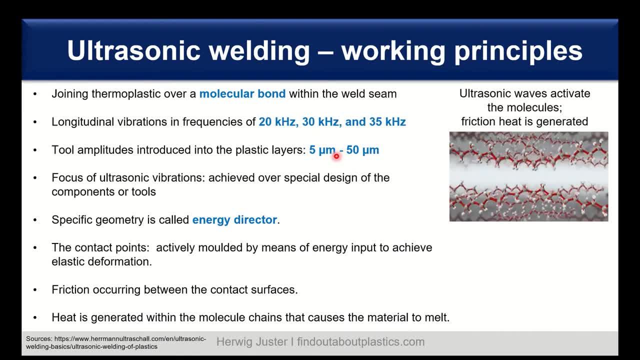 between 5 micrometers and 50 micrometers, and here also to to have a good vibration within the parts, you need a special design of the components or of your tools and the the geometry, the specific geometry which is used, is always called the energy director. 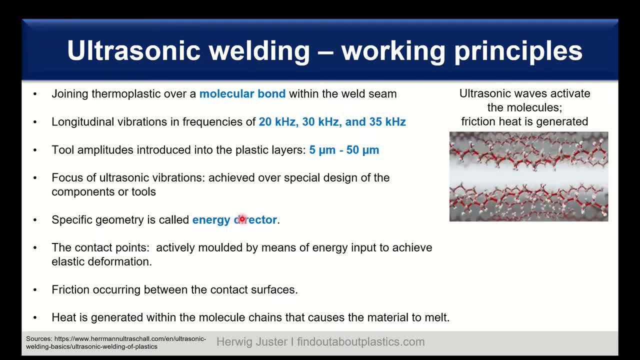 because you need to somehow funnel the waves into a certain direction. but then the basic principle is: we use ultrasonic waves to activate the, the molecules, and they generate in the friction, which results into heat, and with this heat we can cause the material to heat and then generate energy from the waves and the waves that are present in theichi. 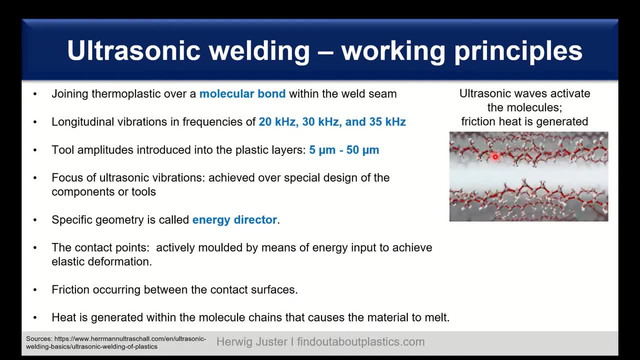 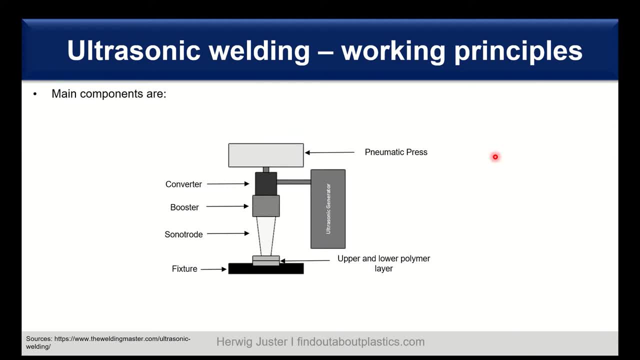 then with the teething, we bond the two parts together. Ok, so how does an ultrasonic device looks like? So here is a schematic representation. So the heart of each ultrasonic welding machine is the ultrasonic generator, which is coupled to a converter and a booster, and the application element is the sonotrode which is then applied. 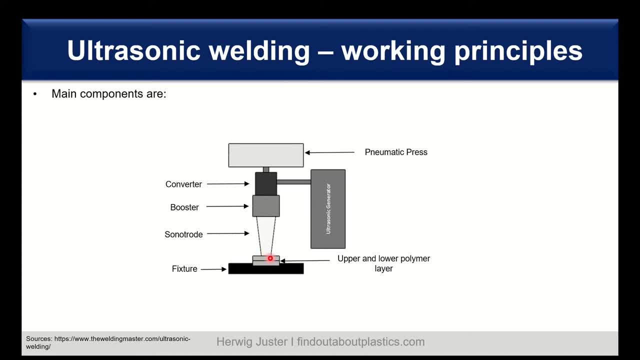 onto the upper polymer layer, and here we have the lower, and those two are melted Then together. we have also the fixture to mount this, and since the sonotrode needs to have direct contact onto the upper layer, we also need a pneumatic press to push the. 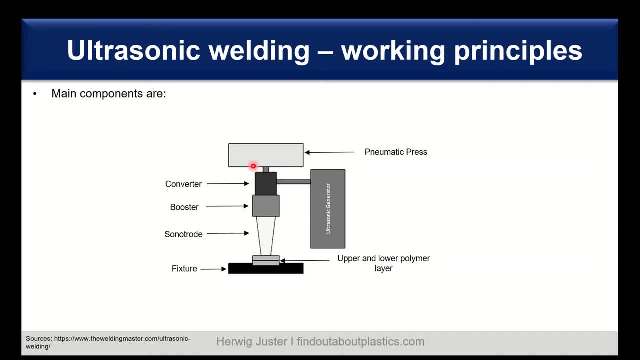 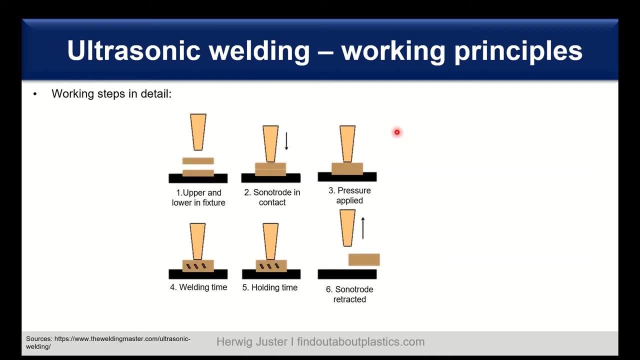 pressure on it to ensure that the waves are guided into the right direction. Ok, let's have a look into the working steps in detail. So we start, we have our fixture, we insert the lower part and then the upper part. Then here we see schematically the sonotrode. 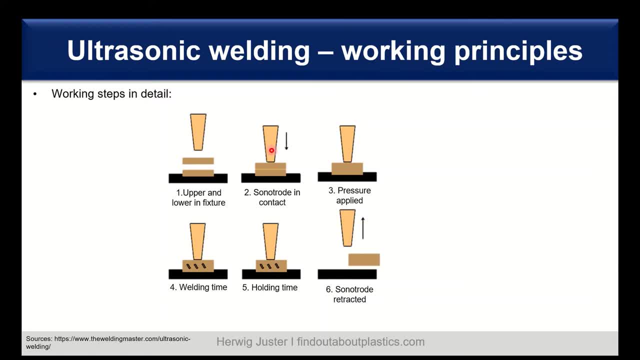 Ok, Then in the next second step, the sonotrode gets in contact with the upper layer, Then we apply the pressure and start introducing the ultrasonic waves, which then result in a friction, so an activation of the molecules, the macromolecules, and then we need a certain 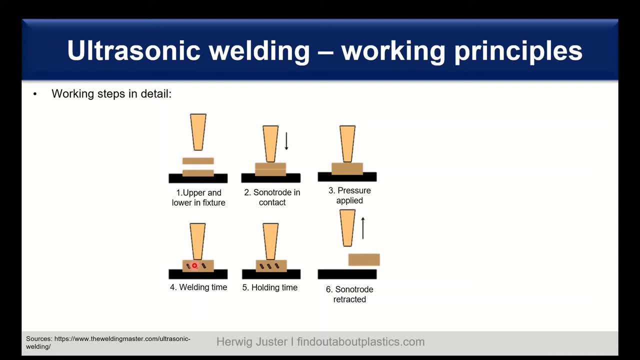 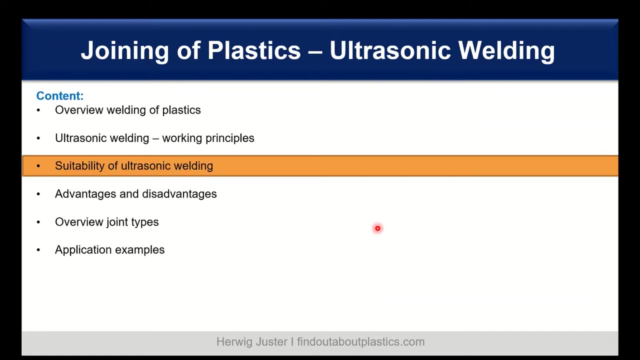 welding time- It's not much, it's a fast process. Then we need to hold it Because we need also to cool down to ensure that we do not lose then the part dimensions also, and after this holding time we retract the sonotrode and have the part welded together. 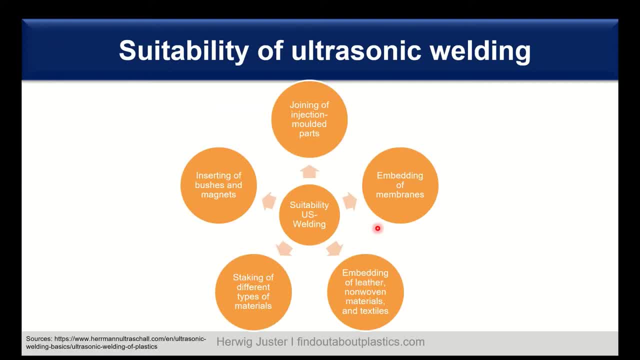 Ok, now we have a look at the suitability of ultrasonic welding. So what we can, what it is mainly used for. So in the plastics industry, in polymer engineering, we use it to join injection molded parts. This is an established state of the art way. 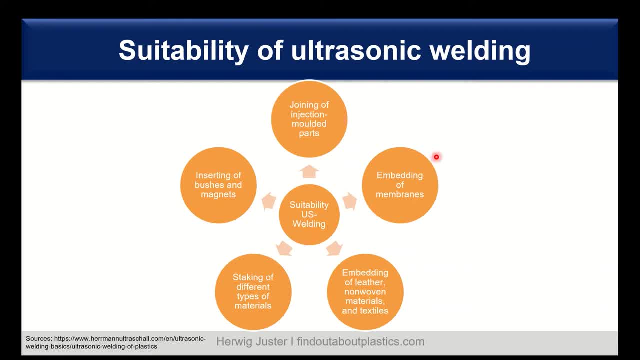 However, there are lots of other possibilities. For example, when you have membranes, you can embed it in a certain plastic frame and weld it, Especially for the medical application of membranes. It's really a clean process, the ultrasonic welding. We can also use other materials, such as leather, nonwoven materials or textiles and combine. 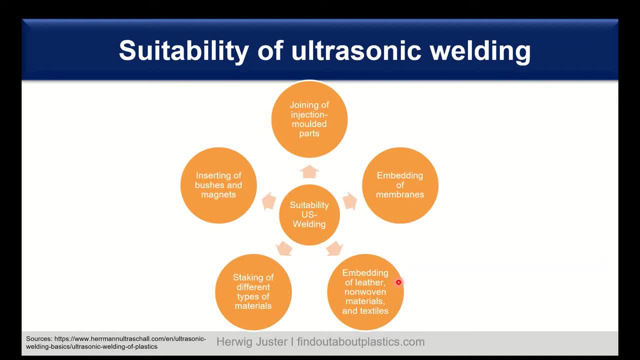 those together and weld them, Or just different type of materials, such as welding a plastic with a leather element, for example. Or we can also insert different kind of materials, Ok, Magnets or other bushing parts to have here, to not have a two component molding. but then 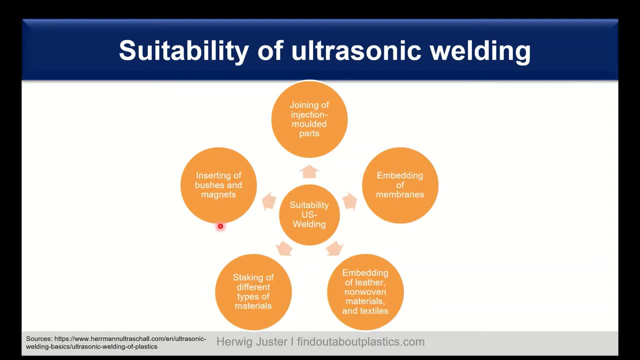 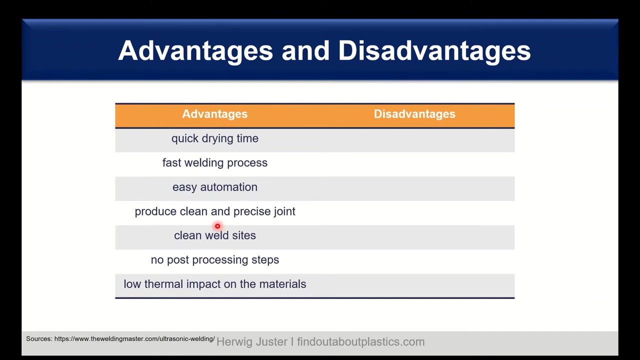 to insert these afterwards and weld it together. So it's a quite versatile welding technique and allow not only plastic materials to be welded but also other materials. Ok, Let's discuss the advantages and disadvantages. So, as a major disadvantage is the quick approach of doing the thing, 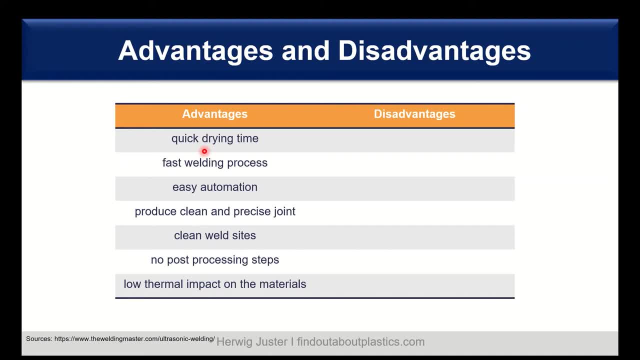 So it's a fast welding and quick trying time. We can easy automate the whole steps. We can produce a clean and precise joint and have clean welding sides itself And we have no problems with the welding And we have no post processing steps involved. 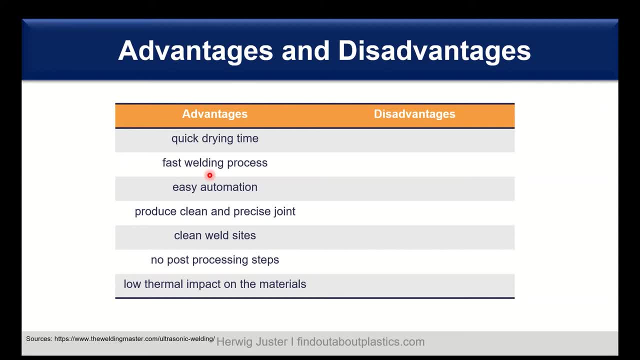 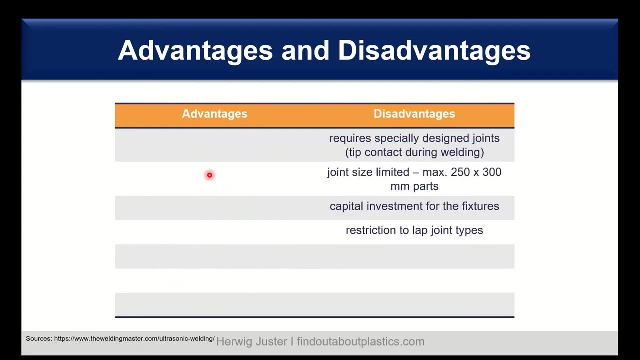 Also important is the low thermal impact on the materials itself. So it's just in a few seconds the welding is completed and have just this inner friction of the parts. Disadvantages, For the focus needs to be given at the joint design itself. 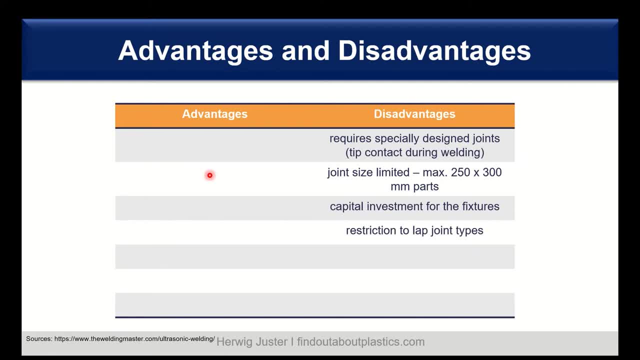 so you need specially designed joints, especially to have a proper tip contact during the welding. then also there are some joint size limitations in terms of parts, what you can weld, and you also need to have some first capital investment for the fixtures but also for the whole device itself. 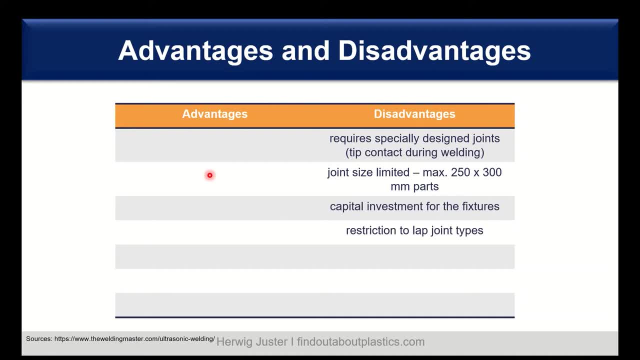 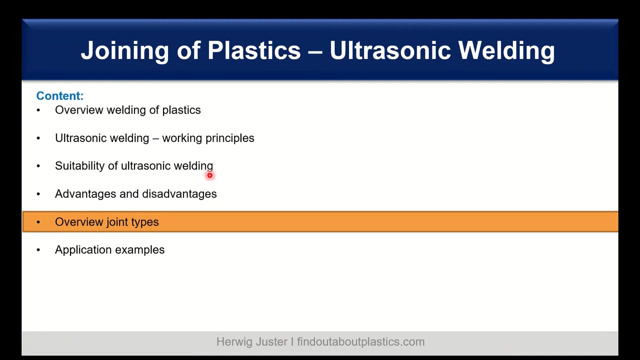 but this is what we also discussed in laser welding. once these initial investments are completed, then it's a, it's a all over, a cheap process. yeah, and there is a restriction to the lab joint types you can, you can fulfill. okay, important part of the ultrasound is the other joint. 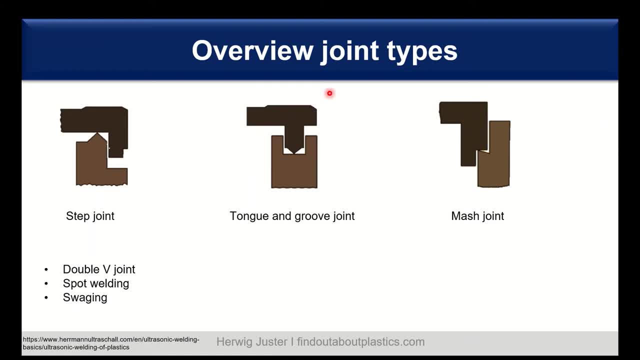 types- and this is what we discuss here now- give an overview of the of some of the joint types. so the most common use is the so-called step joint and it's a advantage is the easy implementation in the injection molding tool. and you see, here the base layer has here this step in and here we place the upper layer and this step will be. 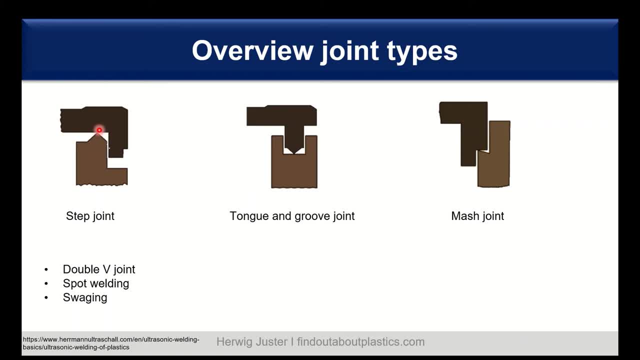 uh by the use of the ultrasonic will be uh molten and then we have here this surface will then attach to here, to this straight surface. then we can achieve here high strength and airtight welds. and the advantage is also it has a self-centering function through this. 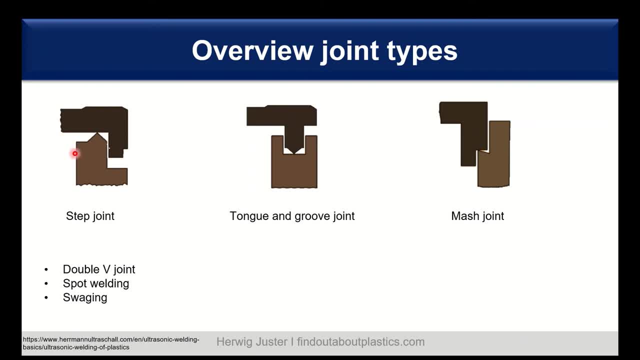 shape and it's, uh, well used also among the amorphous thermoplastics. then we have the tongue and the groove joint. so what you can see here in the base layer we have the, the u shape, which is our groove, and we see here again the, the little step which will be molten. 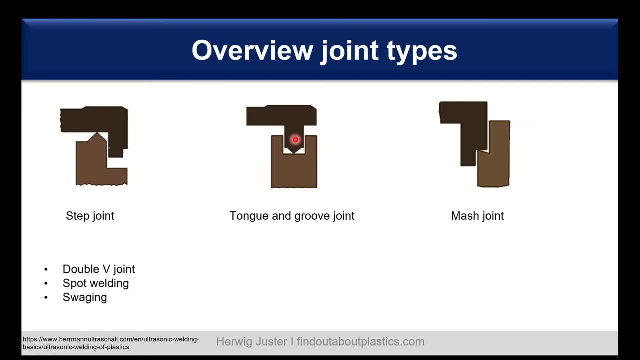 and then attach to the, to the whole tongue, uh, to the whole groove. so this is the tongue, and among all the joint types here we can achieve the, the greater strength and um. also, this gap results in a, in a um, in some kind of capillary effect. so 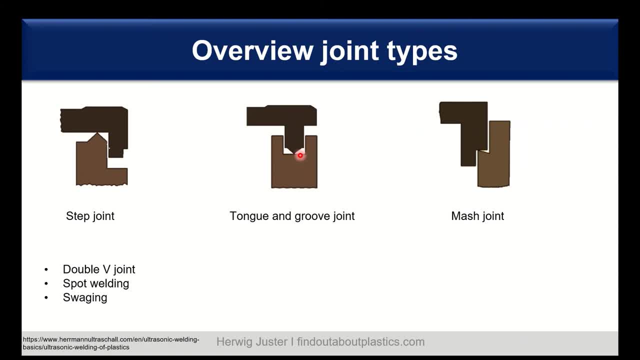 it's really uh soaks. then the the melt in into this uh groove, and this is also one of the reason why this uh greatest strength of this weld is achieved through this capillary effect. uh, then we have the so-called mesh mesh joint. here we can achieve also. 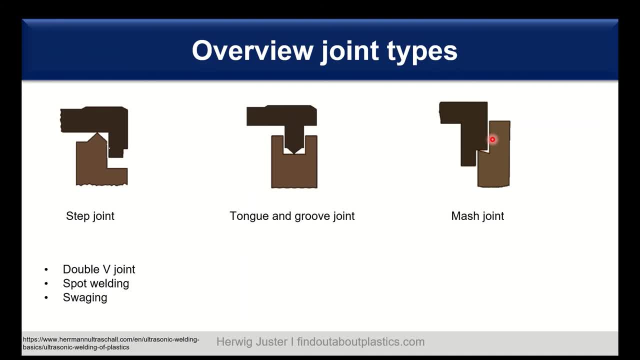 um airtight and high strength weld. uh also for um thin thin walls. uh, this joint is suitable and- and it is also often applied in firmware- semi-crystalline thermoplastics. okay, then there are several other. i just list them here: the double v. 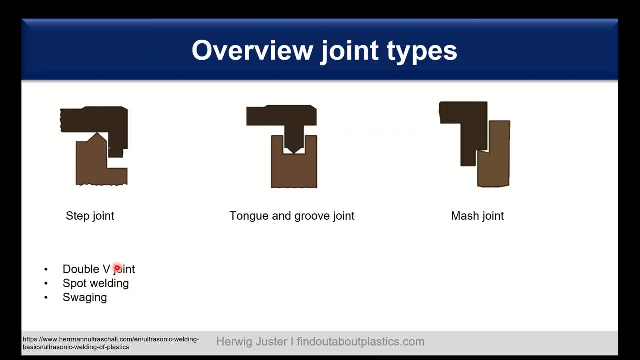 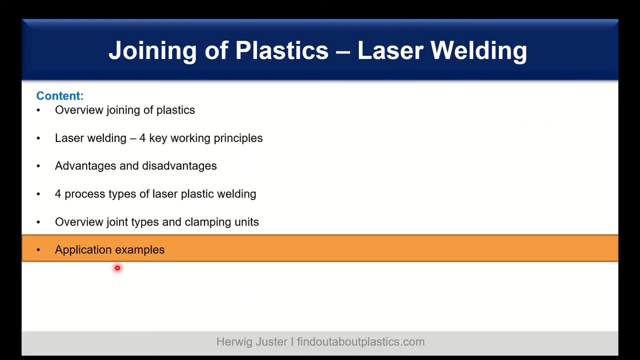 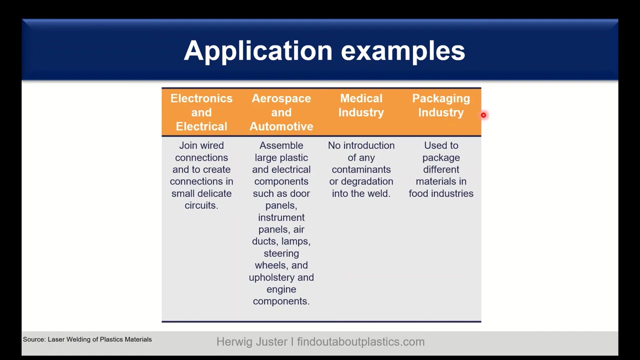 joint, spot welding, swagging. so there are, there are in the literature different type of joints. it's really established, uh, these designs and what you can also deepen them, um, okay, let's finish with the application examples. so here i've selected four different industry, for example electronics and electrical. so here you can join wired connections. 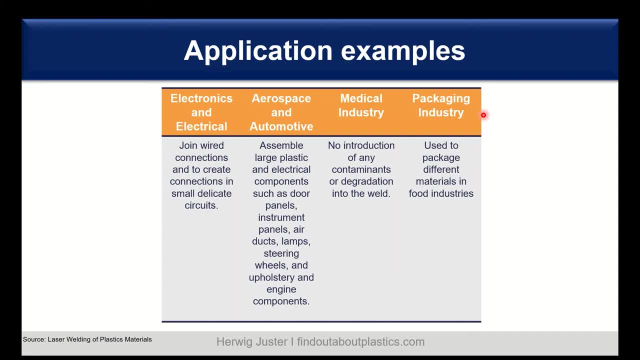 and also create connections in small, delicate circuits. this starts from mobile phones over computers or any other electrical devices, electrical or electronic device in aerospace and automotive. here in automotive, there are the possibility to assemble larger uh, plastic and electrical components, for example, such as the door panels or instrument panels, or also air ducts, lamps, front end lamp and. 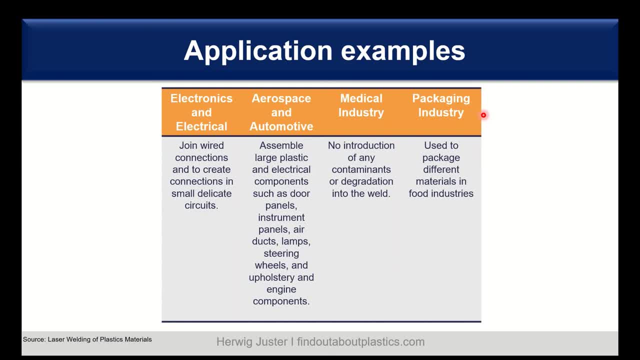 are a good example. there are parts of the steering wheels and upholstery, as well as components which you can um weld with this technique: the medical industry, what we already touched on, the this joint weld is not introducing any contaminations or degradation. there is a major advantage: you want to to avoid to have here some contamination. 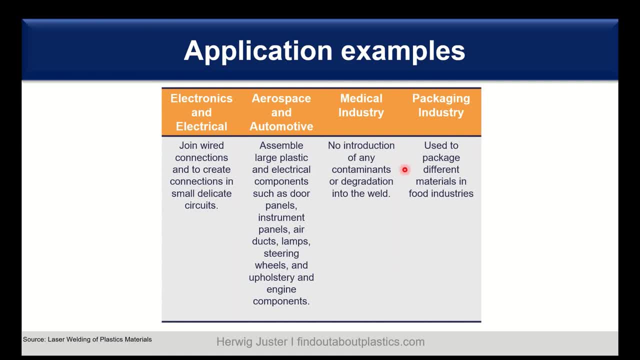 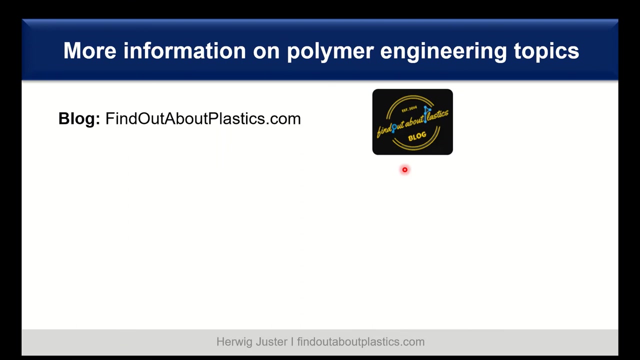 packaging. industry. here it is used to have multi-layer, different types of plastic layers weld together to have a protection towards air or other oxidizing things, to protect the food in the food packaging. More information on different polymer engineering topics can be found on my blog, findoutaboutplasticscom. 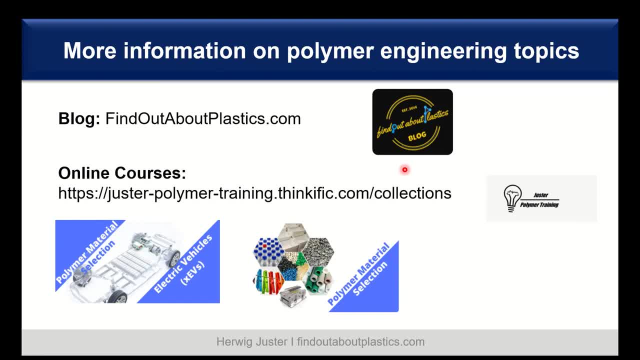 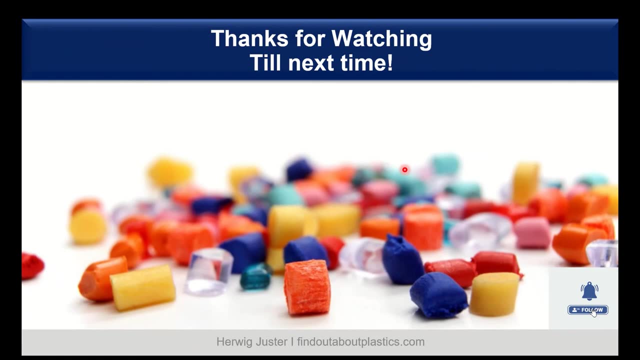 and also I offer online courses for polymer material selection. I will link you both the blog and the online courses in the description below. Ok, thank you for watching and do not forget to subscribe and smash that like button. Till next time and bye.